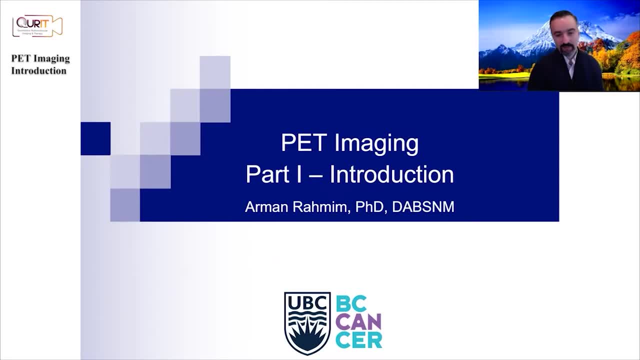 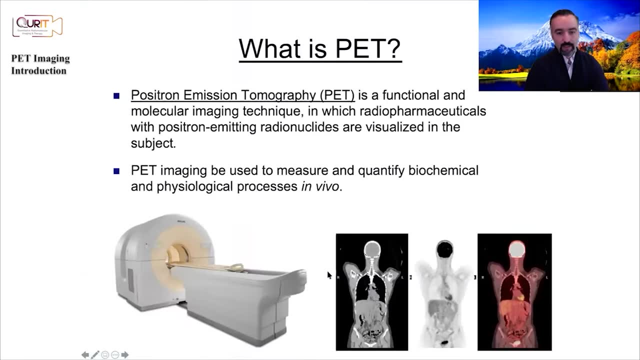 technology and practice and art of PET imaging. So we're going to begin with an introduction here. So what is PET Standing for positron emission tomography? It's a functional and molecular imaging technique where radiopharmaceuticals with positron-emitting radionuclides are visualized in the subject that 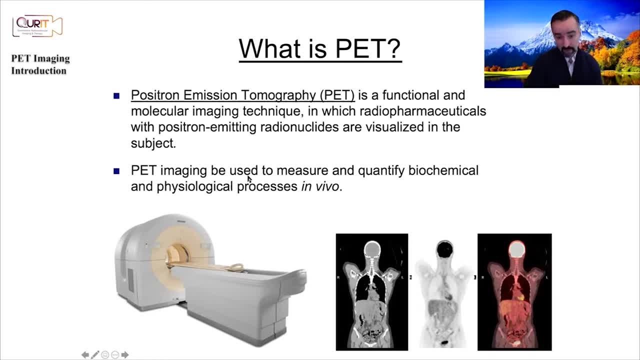 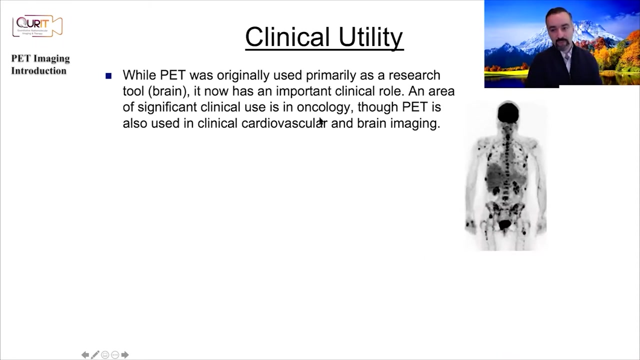 is being scanned, And PET imaging can be used not just to visualize but also to measure and quantify processes- biochemical and physiological processes- in vivo. So PET has. originally, PET was envisioned as a research tool, particularly for the brain. That's where fluorodeoxyglucose, FTG-PET, was used and we're going to talk about that. But it's really 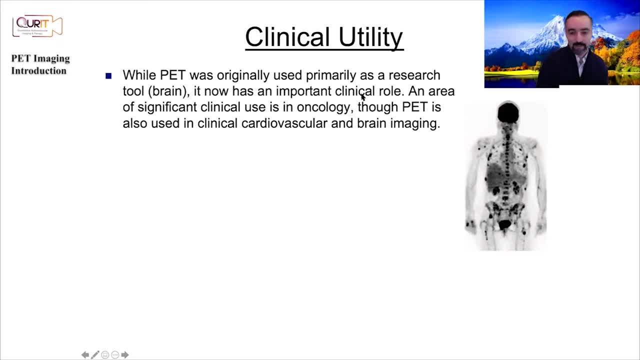 found important routine clinical applications beyond research. continues to be used extensively for both clinical imaging and clinical um tasks and also research oriented studies, and an area of significant clinical use has been in oncology. continues to be in oncology, though pet is also used in other clinical uh frontiers, such 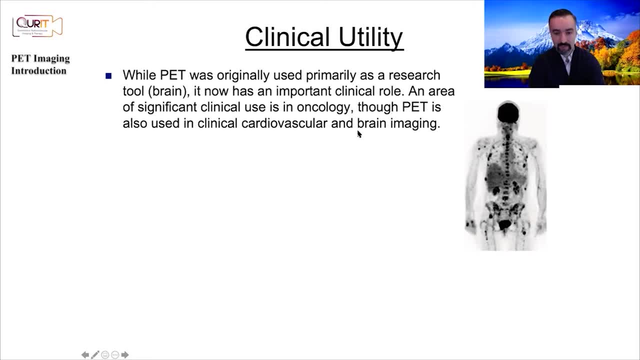 as cardiovascular and brain imaging, especially with the emergence of amyloid imaging, for example, looking at alzheimer's disease. the most widely used radio tracer or radiopharmaceutical has been the so-called fluorodeoxy glucose radio, labeled with fluorine 18.. it follows a similar metabolic. 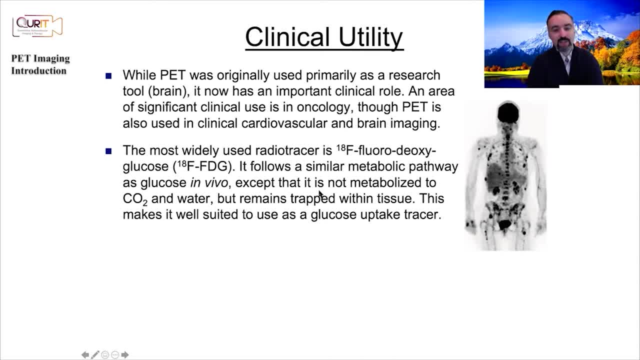 pathway as glucose in vivo, except that it is not metabolized, you know all the way, and gets trapped within tissue- and we will see this shortly- and that's an advantage because it would accumulate, for example, in the tumors and this makes it really well suited to use as a glucose uptake radio tracer. 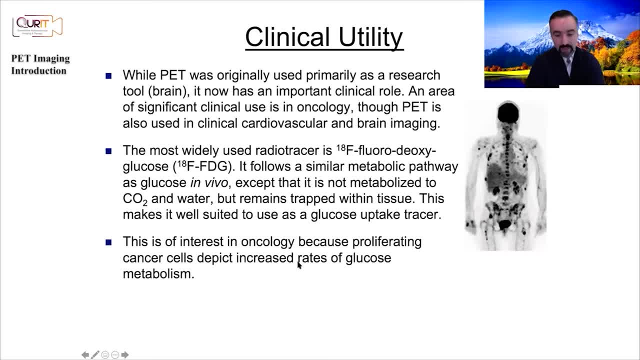 and this is especially of interest in oncology, for example, where you know cancer cells that are proliferating, they're going to be depicting increased rates of glucose metabolism. you sort of might be seeing in this image, so you sort of think of it as it's a glucose analog sometimes. 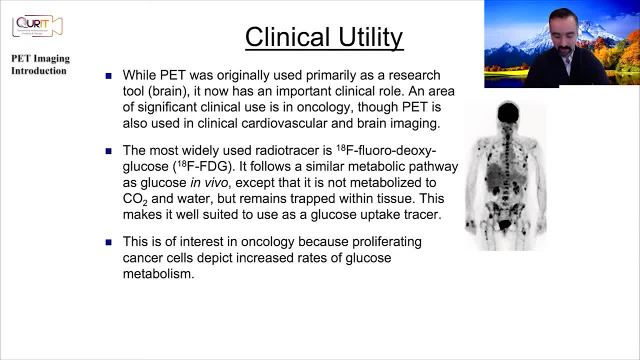 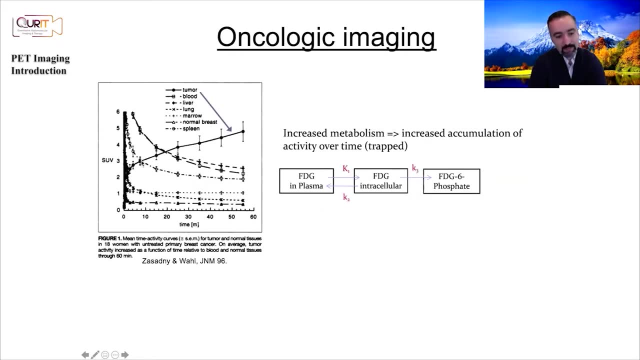 sort of to. to use just a simplified language, we call it radio labeled sugar. it is a glucose analog. it behaves like glucose and basically allows you to visualize and quantify metabolism as such. so here's an example of, for example, how the standard uptake value in the image, which is essentially the 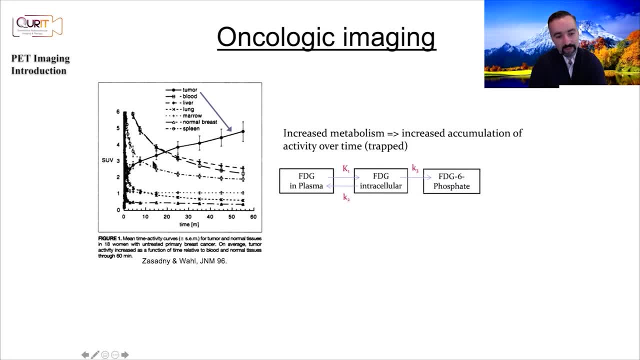 you know the numbers that you get in the image as a function of time, how they grow. this is a metric that we will visit in the future. it's a normalized metric. a value of one represents sort of background images, and values more than one depict higher metabolism. so you sort of see that. 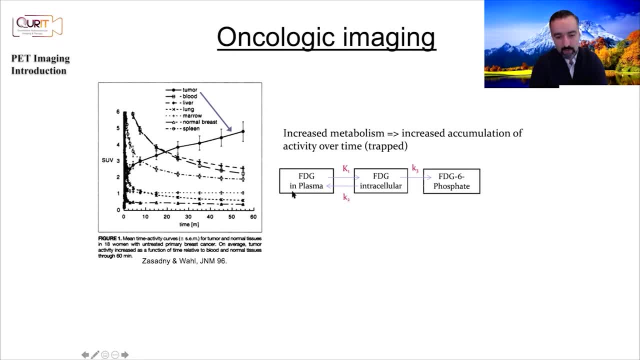 as you inject it. fluorodeoxy glucose is first in the plasma, in the blood, then it enters tissue and into the cells and after that it there is this process of phosphorylation, where you have fluorodeoxy glucose, six phosphate, but the point is- and this is the accumulation, if 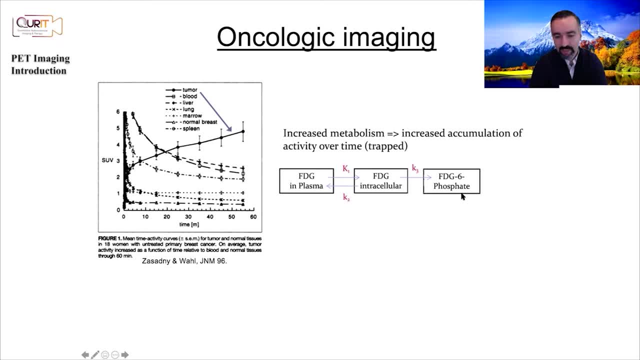 you have increased metabolism, such as in tumors, you have increased accumulation, and the k4 here is assumed to be, and measured to be, very small. sometimes it's just totally ignored, but the point is it's very small. so you have an accumulation of fluorodeoxy glucose. that's what why you have in a 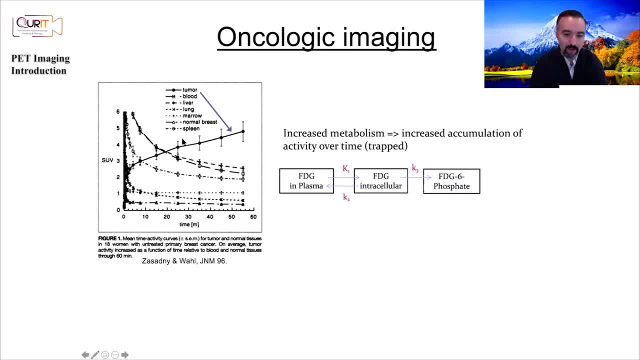 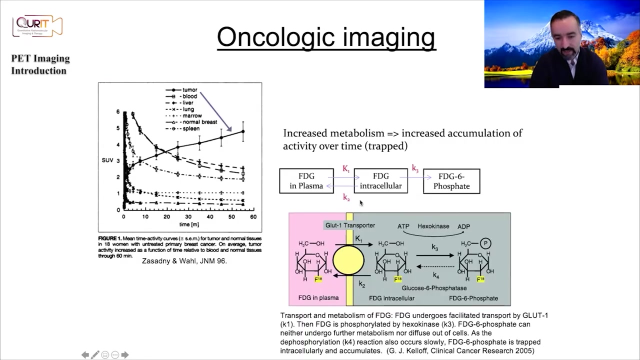 tumor. it keeps accumulating, keeps accumulating, accumulating because you have high rates of metabolism, whereas in other organs, in a good number of other organs, it has an initial uptake because the blood is in the cells, but then it, you know it is entering the cells through this mechanism, but it is then leaving as the blood is cleared from fluorodeoxy glucose, and so this is just a. 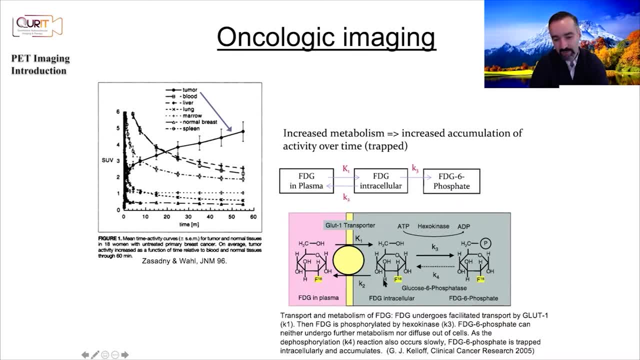 chemical. you know detailed description of what i just told you there. but again, essentially you have fdg plasma- this exact same here, but then here it's phosphorylated and this is where it's trapped. And when it gets trapped, it is trapped within the cells and it is accumulating when you have higher rates of. 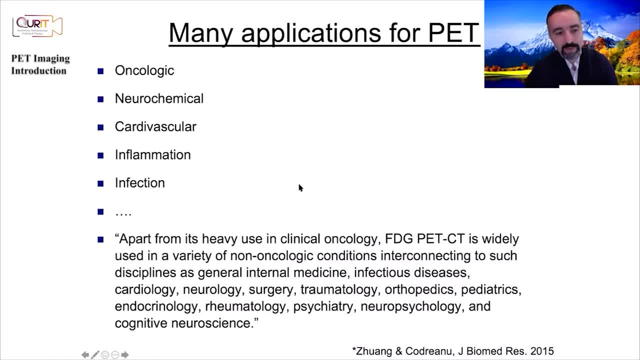 metabolism. Now there are many applications for PET, as we've alluded to. So it's not just for oncologic imaging of cancer, but it's also in looking at neurochemical processes in the brain. For example, you've got cardiovascular imaging. You could be imaging inflammation with it. 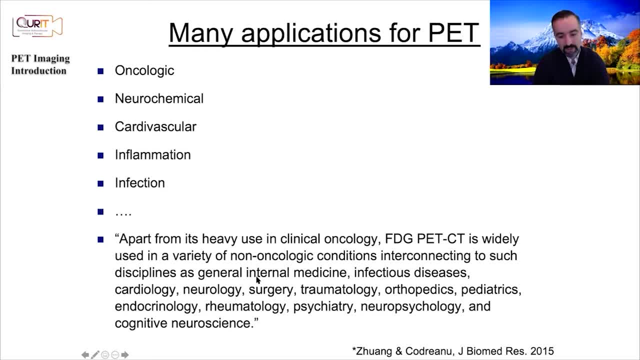 infection with it, many, many, many different things. So I kind of like this statement here that kind of allows you to capture what's going on. Apart from it's heavy use in clinical oncology, fluorodactyl glucose, PET-CT, let alone PET in general. right, This is just for FTG, but even 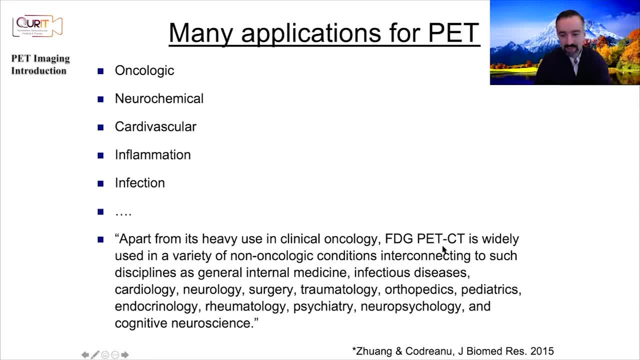 PET in general has even wider applications, But even FTG PET is widely used in a variety of non-oncologic conditions Interconnecting to such disciplines as general internal medicine, infectious diseases, cardiology, neurology, surgery, traumatology, orthopedics, pediatrics, endocrinology. 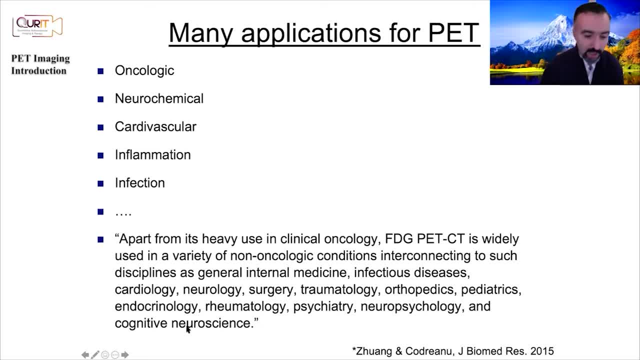 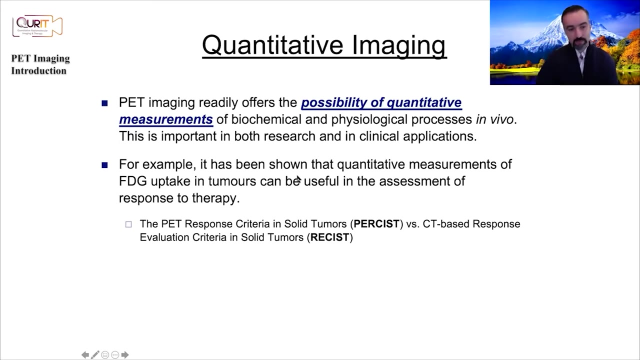 rheumatology, psychiatry, neuropsychology and cognitive neuroscience. So it's just an amazing range of applications that PET and specifically FTG PET have seen. But again, PET imaging has a wide range of clinical and research And the other thing is quantitative imaging, which in a future lecture we will talk about. 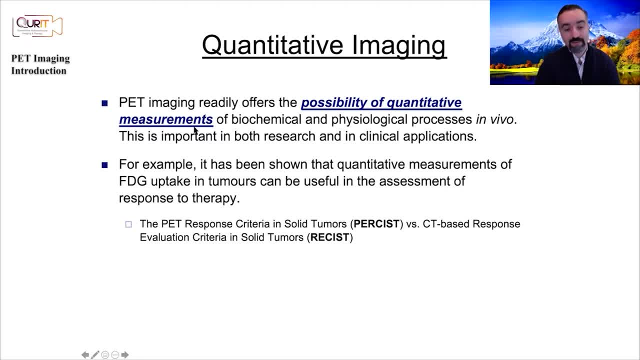 But PET imaging allows you to do quantitative measurements of biochemical and physiological processes in vivo, And this is very important in both research and also in clinical applications, finding more and more applications. For example, it has been shown that quantitative measurements of FTG uptake in tumors can be useful in the assessment of response to therapy, So this is a 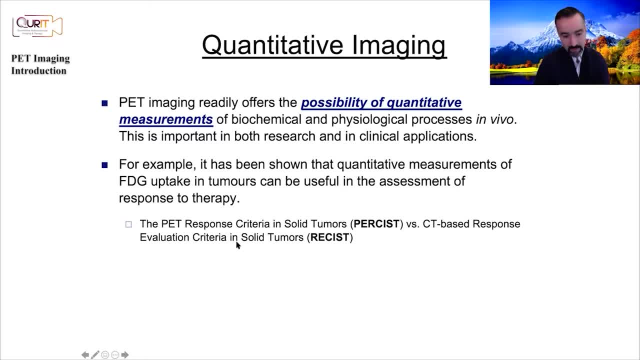 So traditionally you might have heard of this thing: CT-based response evaluation criteria and so the tumors widely used. you know there's been a lot of interest in the past years on this thing, for example. This is just one example, but using PET essentially to assess response to. 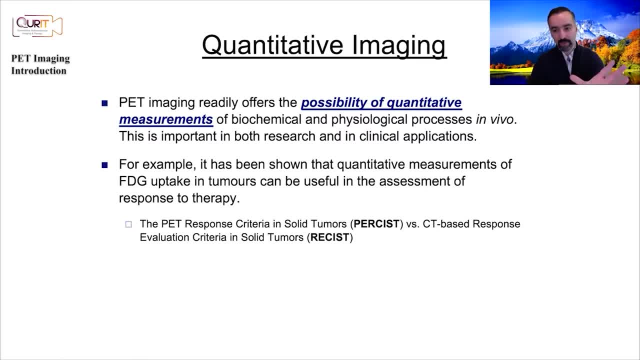 therapy, Let's say, if a patient is undergoing chemotherapy. if you do PET imaging before and after therapy and looking at the numbers, does that allow you to better assess, better assess whether the treatment is working or not, And that would that allow you to better. 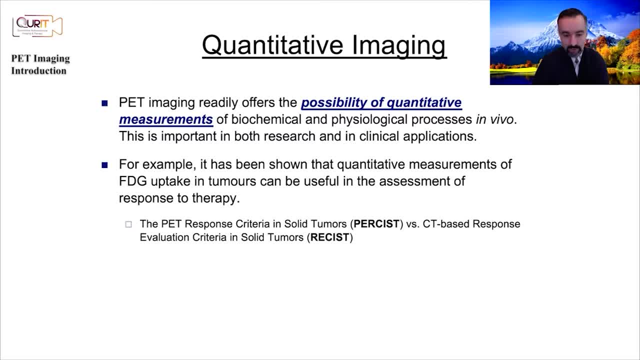 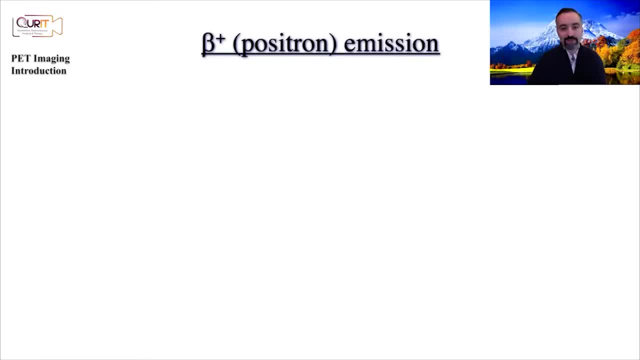 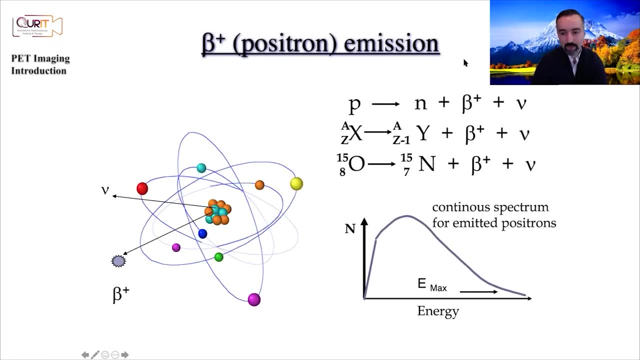 modify and plan for future therapies. So let's talk about some of the fundamentals and the physics of pozitron emission, because at the end of the day, that's what it stands for: positron emission tomography. So let's see what positron emission is about. 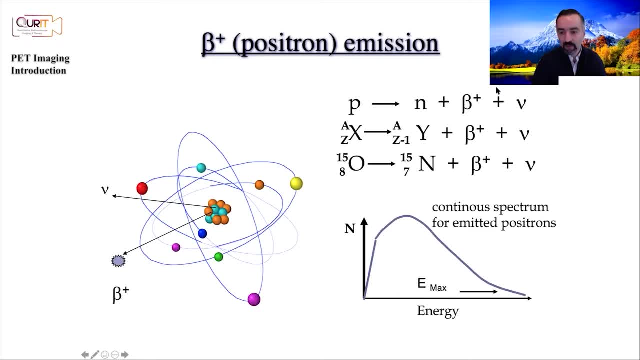 Again. in some of the earlier lectures, Carlos has talked about some nuclear reactions, etc. but this one is the one that we're going to focus on today, where you have a parent radionuclide that emits to a daughter radionuclide and in this process, 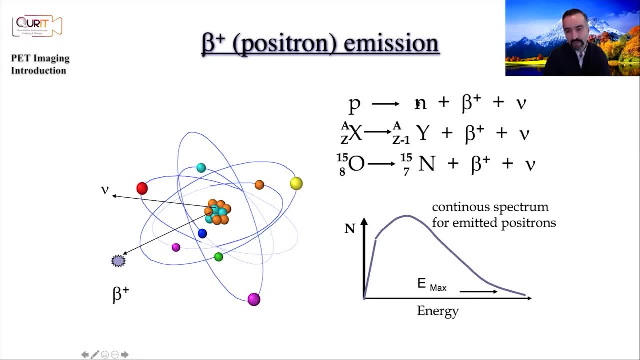 a positron is emitted and essentially you have a proton that has been changed to a neutron. that's what happens. so that's why the total atomic number, um the sorry, the total atomic mass- remains the same, but the atomic number you sort of see goes down right, because you've lost the proton but you're gaining a transit atomic mass remains the. 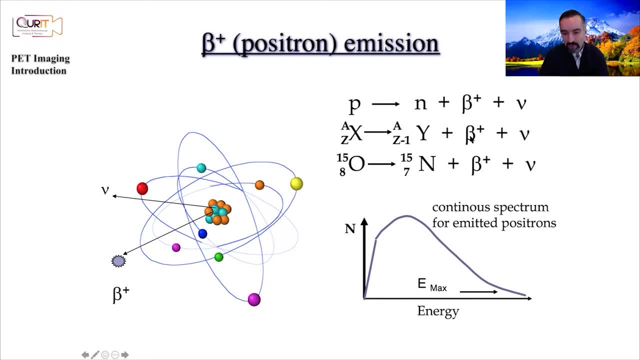 same um, and so you, you emit a positron and a neutrino. we don't image the neutrino. it's very hard to to to measure neutrinos there's. that's a whole frontier on its own. but the only real practical implication of the fact that neutrinos are emitted is that the final kinetic energy of 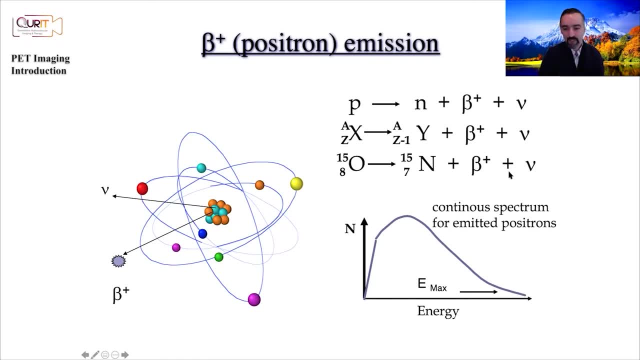 the positron and the neutrino is shared between the two of them, so the positron could be emitted with a range of energies, with a range of kinetic energies, so it's not possible to predict you know which one are we going to get here, but you can get a range of positron emission energies and 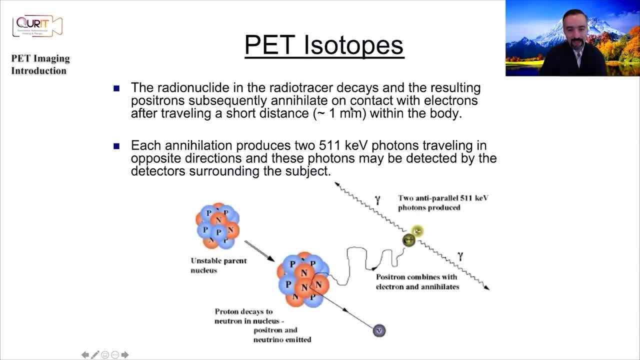 then what happens after that? well, so after that, um, the positron travels a little bit within tissue and it is slowed down. okay, so it's kinetic energies, it could be high. it is slowed down and finally, um, it annihilates in combination with electrons. okay, so it is slowed down. this is called a positron range, okay, so this, this could be for. 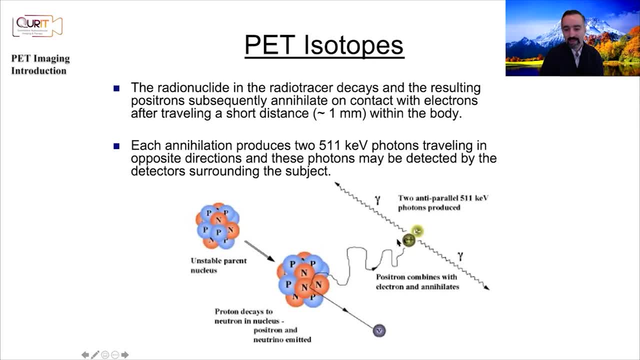 example, a positron range, and then it's slowed down, and then it's slowed down, and then it's going to be, for example, let's say, half a millimeter, okay, and then finally you have the positron and an electron. the two of them annihilate the classic equals, mc squared, the entire rest mass. 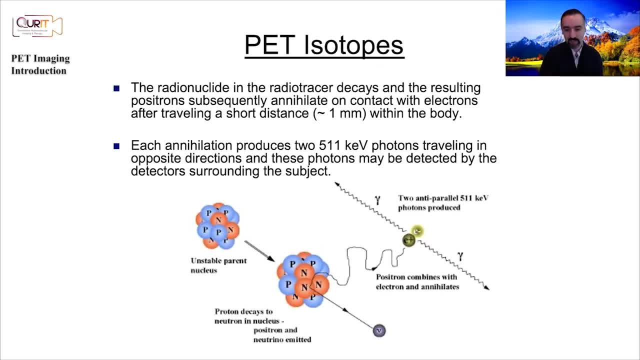 is lost to two gamma rays in opposite directions- anti-parallel- and the rest mass of of an electron and a positron each is 511 kv, so that's going to be the energy that you're going to get for these two anti-parallel gamma rays. 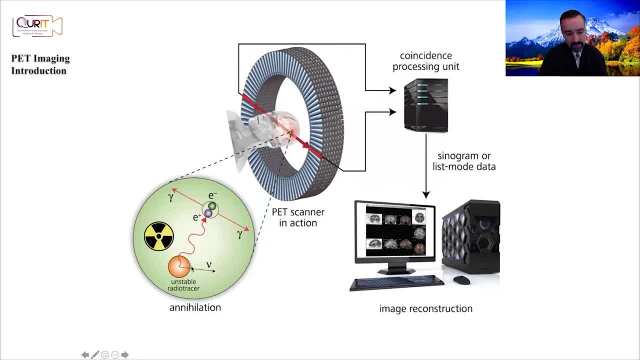 okay, and so this is again just showing the same thing, where you've got the positron after a small positron range- again sub millimeter, typically for for fdg, for fluorine 18, but could be more than a millimeter for other radio tracers- and then after that you've got these two anti-parallel gamma rays. 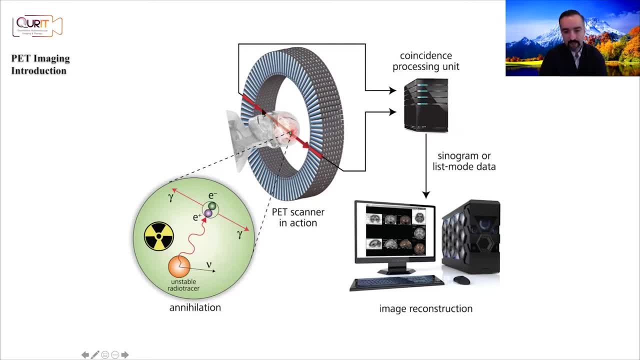 and um. then you get these two photons and you have detectors all around the patient, for example- that are able to say: hey, wait a minute, i got an event here, i got an event. these are arriving at almost the same time. therefore, these must correspond to the same event. therefore, i can. 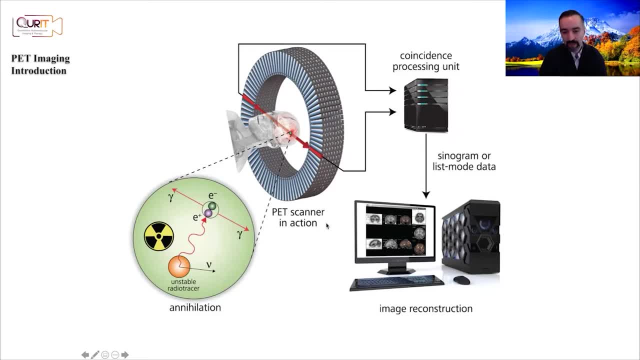 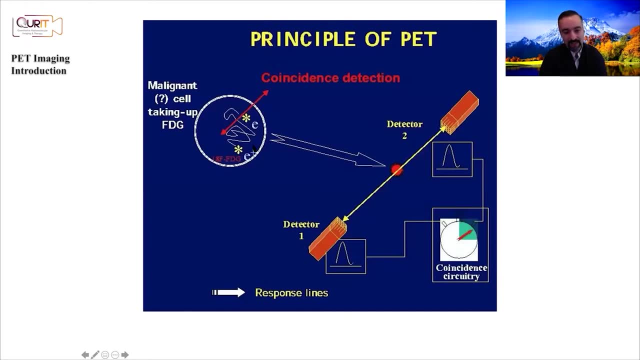 draw a line of response and so you do that. so we're going to talk in more details, but again in the context of, let's say, fdg, you might have a malignant cell that is taking up fdg more than other um tissue in the body. it is emitting and you've got detectors around it and it is able to. 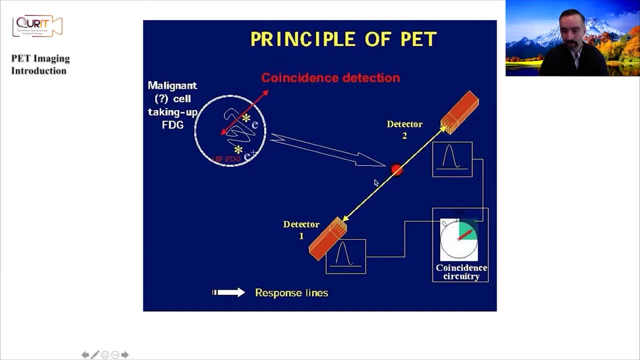 draw a line of response saying: i've got an event here, i've got an event here, i've got an event here somewhere, from somewhere along this line. now, you don't know from where exactly, along this line, but at least you can draw a line. and that is very good because, as we've talked about before in the 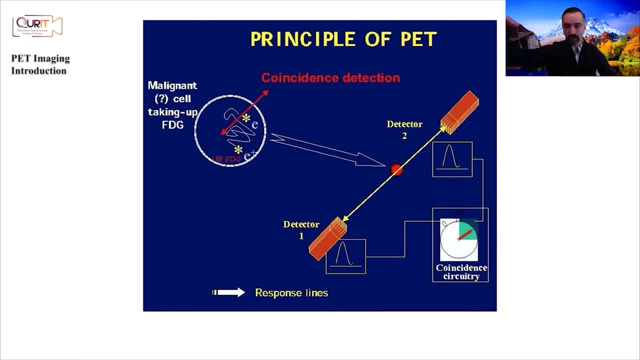 context of tomographic image reconstruction. if you're able to get projections of your radioactivity at different angles- and you have that, those collection of angles collected- then you can do tomographic image reconstruction and you can actually reconstruct where this event came from from a single line of response. you don't know where this event came from, so the more you can. 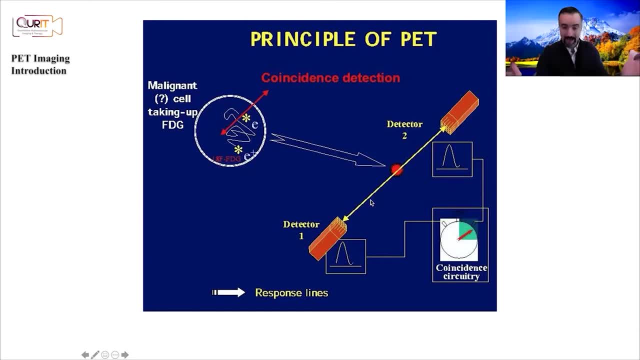 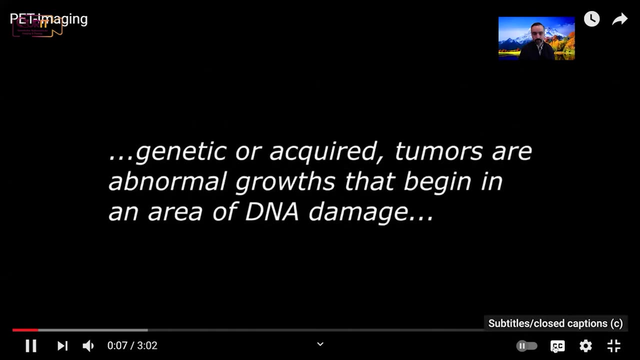 is along this line. but if you acquire a look you know around the patient, then you can do image reconstruction and reconstructing image. so let's look at a couple of videos here. imaging helps us find cancers in the body, be it genetic or acquired. tumors are abnormal growths that begin in an area of dna damage. 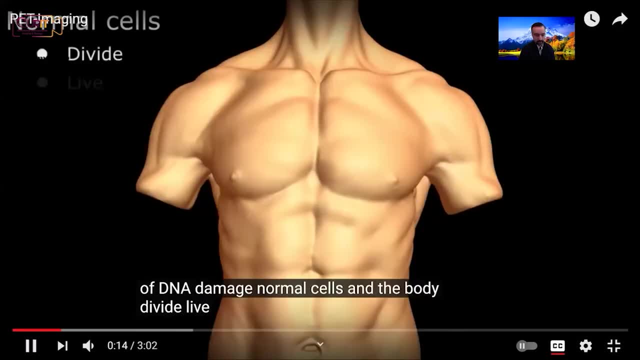 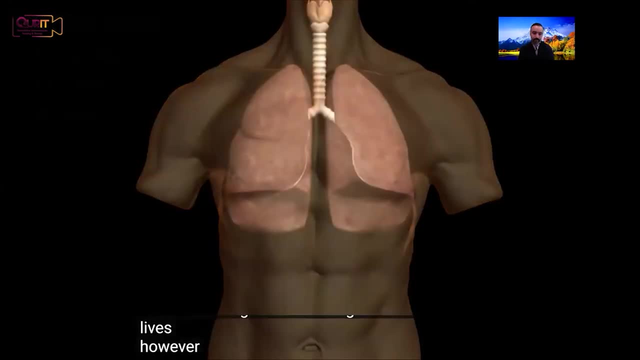 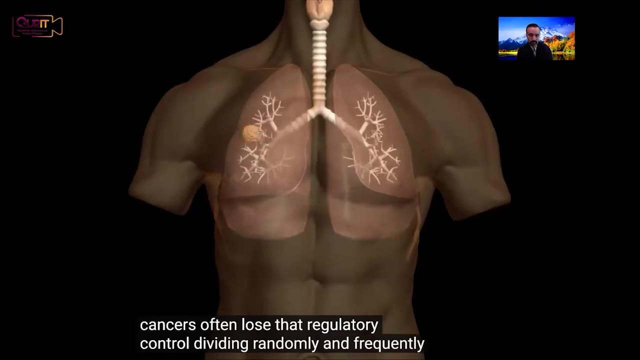 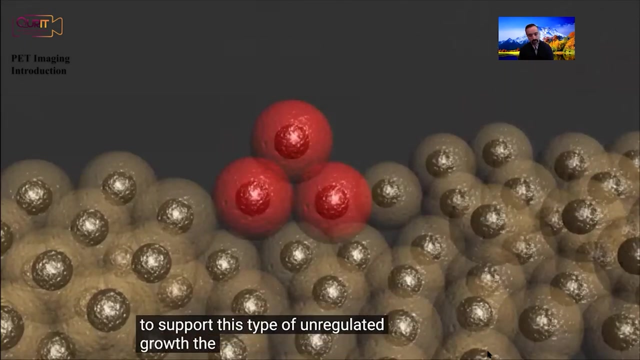 normal cells in the body divide live and die in a tightly regulated process that ensures our tissues and organs last throughout our lives. however, the genetically damaged cells of cancers often lose that regulatory control, dividing randomly and frequently to form a tumoral mass or lump. to support this type of unregulated growth, the tumor cells metabolism is upregulated. 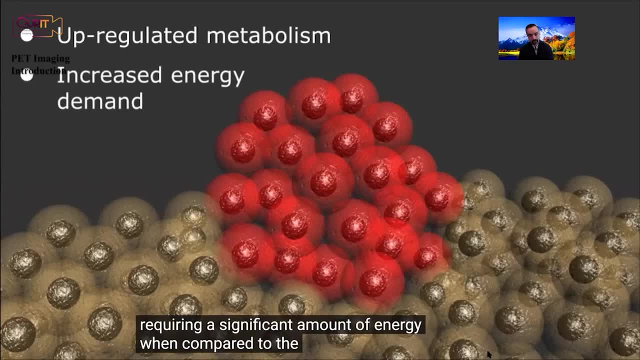 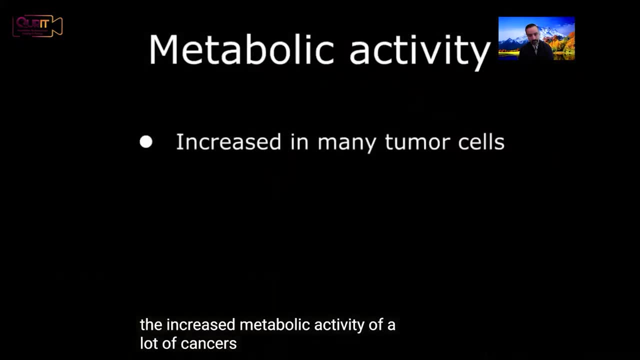 requiring a significant amount of energy when compared to the normal surrounding tissues. the increased metabolic activity of a lot of cancers is a significant amount of energy when compared to the normal surrounding tissues and a significant amount of energy when compared to the normal surrounding tissues. key feature of tumor cells that can help us distinguish them from the normal surrounding. 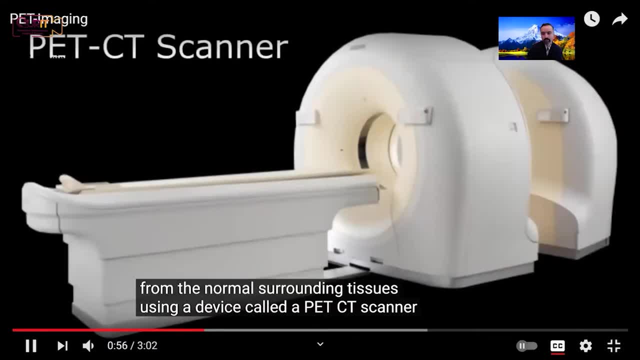 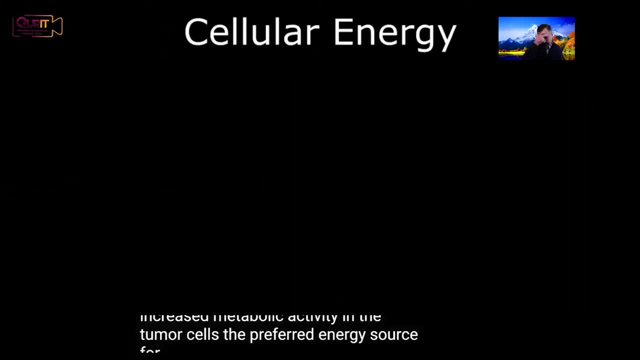 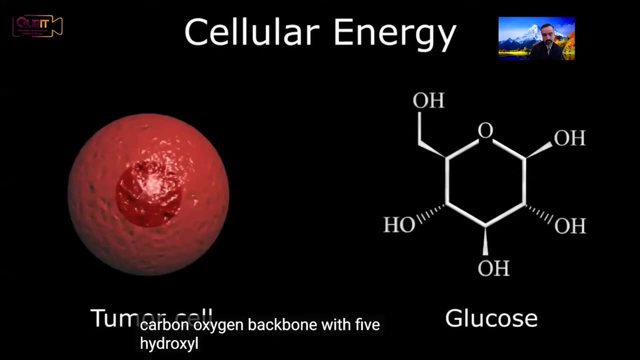 tissues. Using a device called a PET-CT scanner, we can actually see and document this increased metabolic activity in the tumor cells. The preferred energy source for tumors is glucose, the basic carbohydrate consisting of a hexagonal carbon-oxygen backbone with five hydroxyl side. 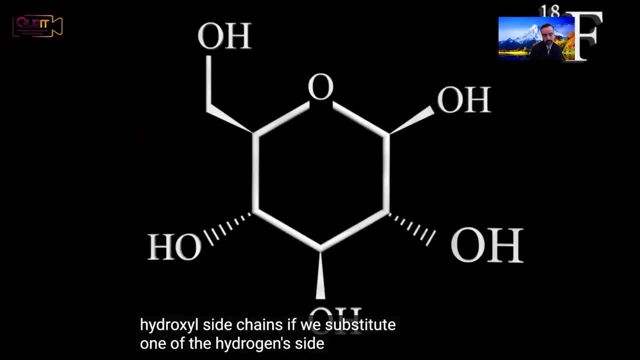 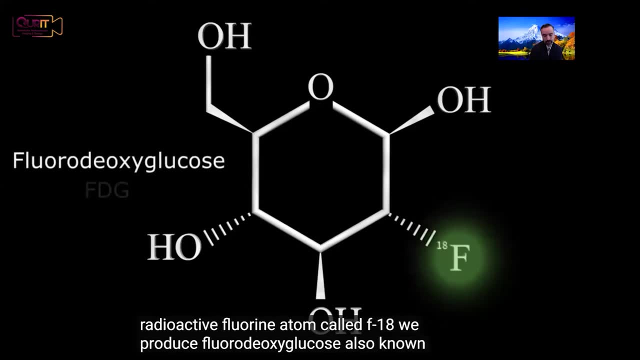 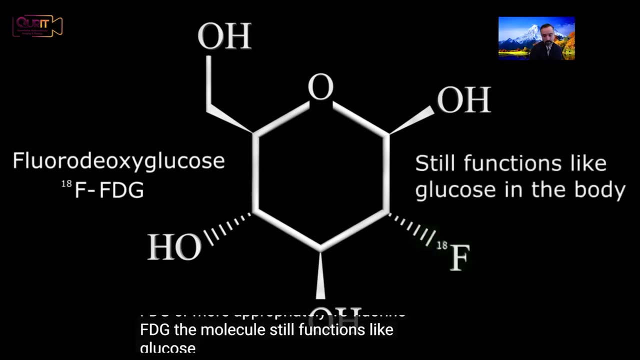 chains. If we substitute one of the hydroxyl side chains with a radioactive fluorine atom called F18, we produce fluorodeoxyglucose, also known as FDG or, more appropriately, 18-fluorine FDG. The molecule still functions like glucose in the body and is therefore known as a glucose analog. Now let's take a closer look at the fluorine 18 atom. The only stable isotope of elemental fluorine is fluorine 19, with nine protons and 10 neutrons. The isotope fluorine 18 is created in a cyclotron and still contains nine protons. 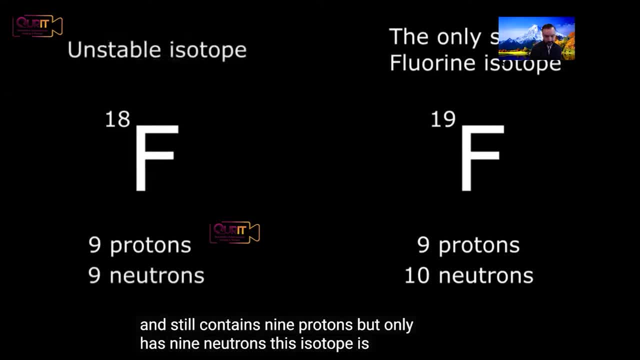 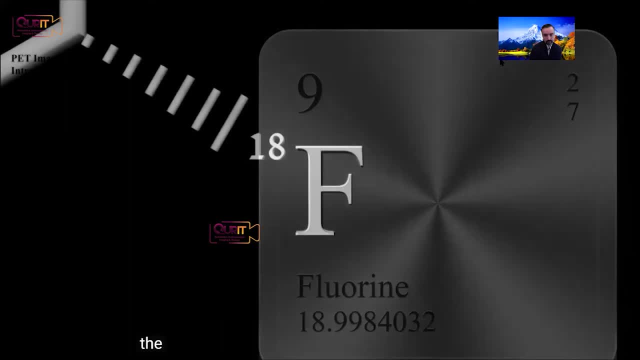 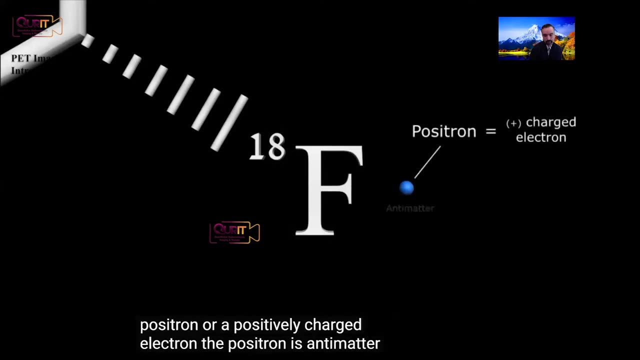 But only has nine neutrons. This isotope is unstable and therefore undergoes radioactive decay. The radioactive fluorine atom emits a positron or a positively charged electron. The positron is antimatter and therefore quickly collides with a nearby negatively charged electron. 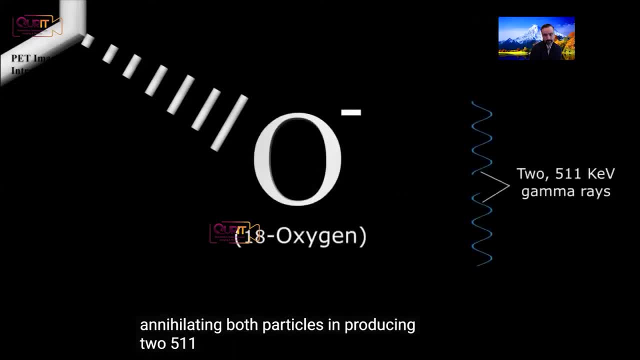 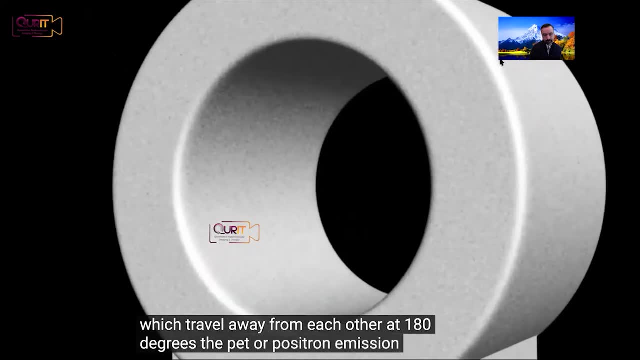 annihilating both particles and producing two 511 kiloelectron volt gamma rays which travel away from each other at a rate of 1.5 to 1.5.. The positron emission tomography scanner can detect these gamma rays and determine where. 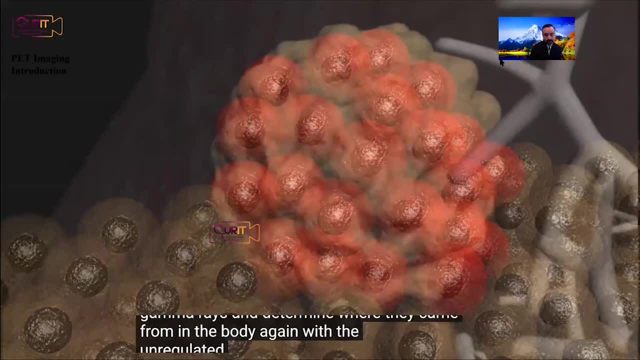 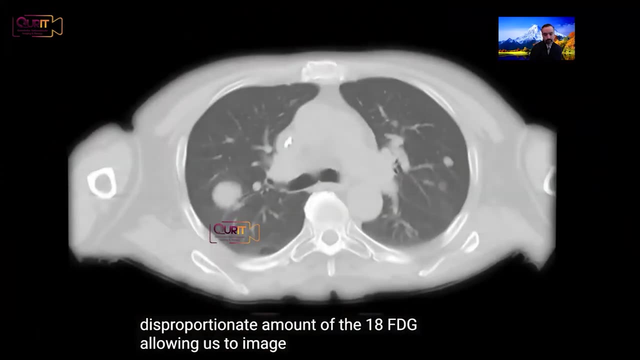 they came from in the body. Again, with the unregulated growth of some of these tumors, the cancer cells will pick up a disproportionate amount of the 18 FDG, allowing us to image this activity on the PET scanner: Tissues that have an increased metabolic activity and use a lot. 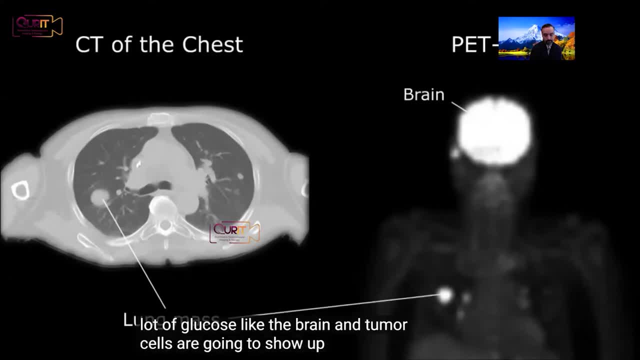 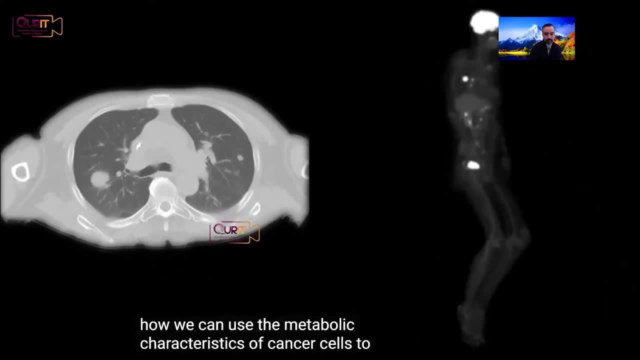 of glucose, like the brain, and tumor cells are going to show up bright on the PET image. So that's a quick example of how we can detect these gamma rays. We can use the metabolic characteristics of cancer cells to find tumors in the body. 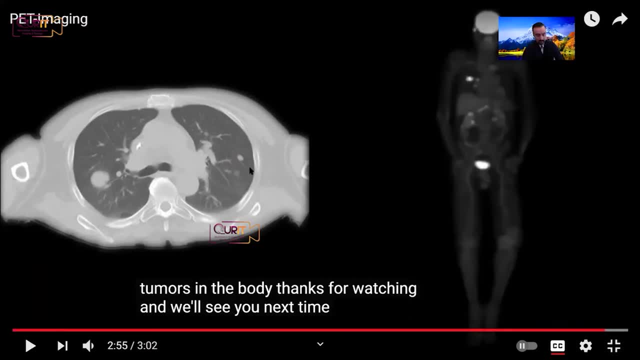 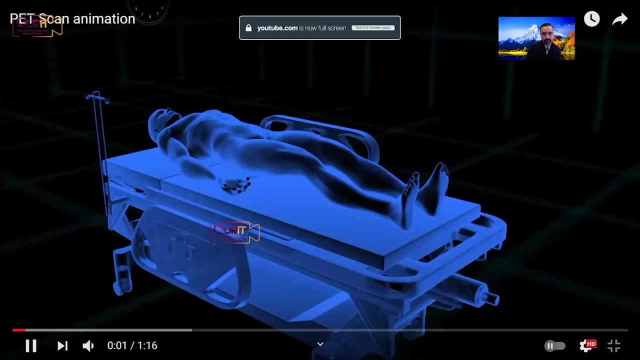 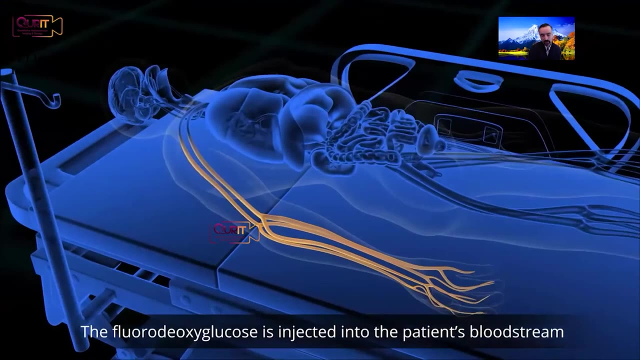 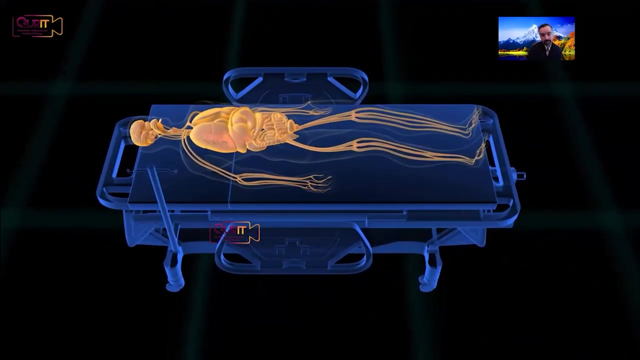 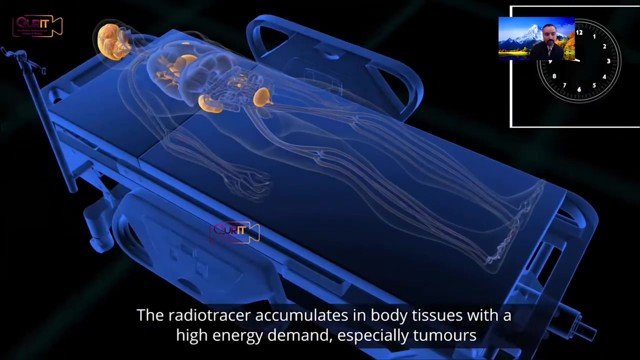 Thanks for watching and we'll see you next time. Picking up by the cells, but then those with higher metabolism, for example. but let's say the brain is a place where there's a lot of metabolism going on, so you'll see it. but also. 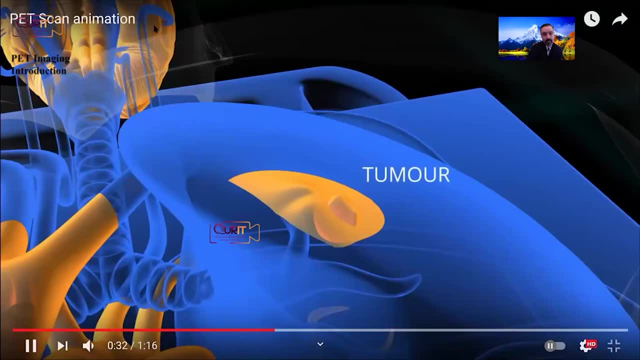 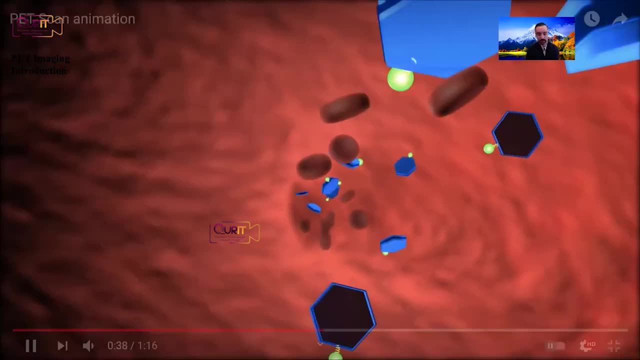 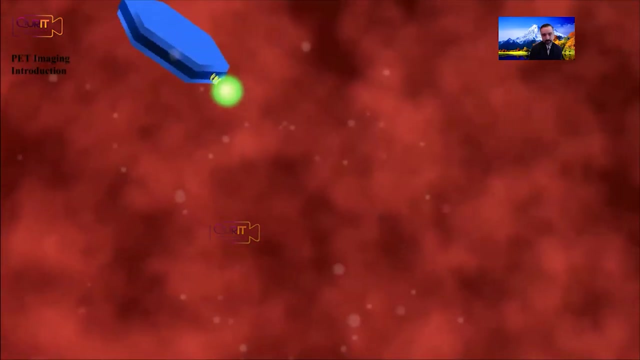 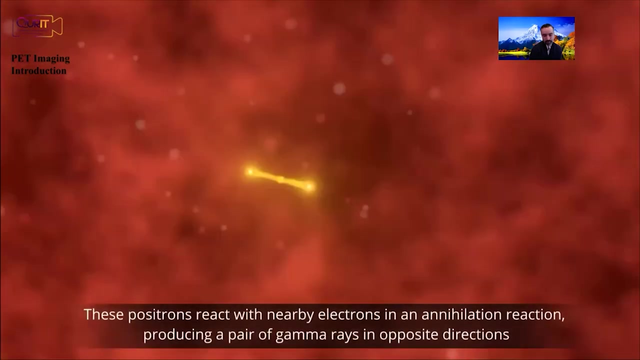 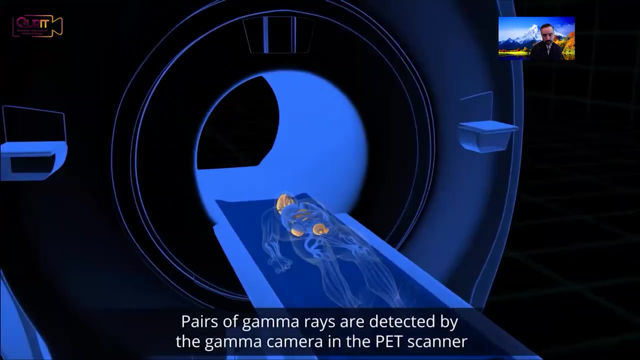 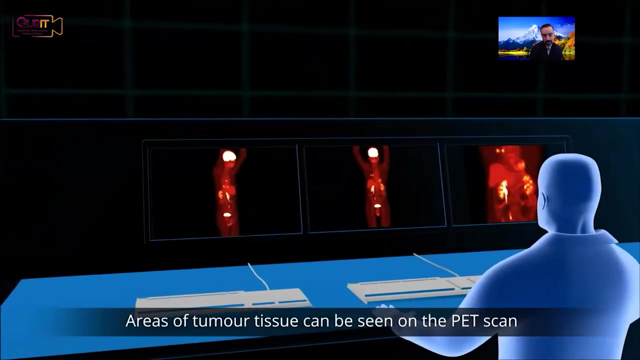 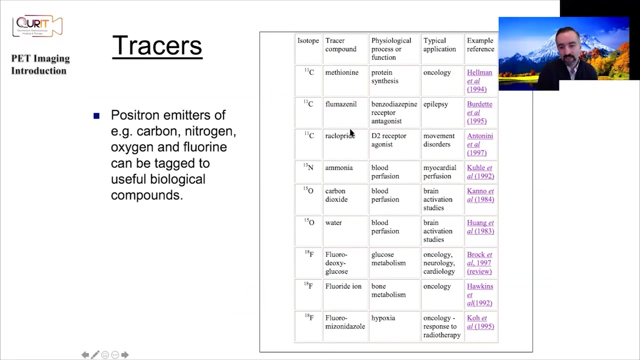 in tumors, for example. So this would be normal uptake in the brain, but also here we have abnormal uptake And a clinician is trained to distinguish between normal uptake versus abnormal malignant uptake. Just some examples of many, many different applications. Again, these are very, for example, 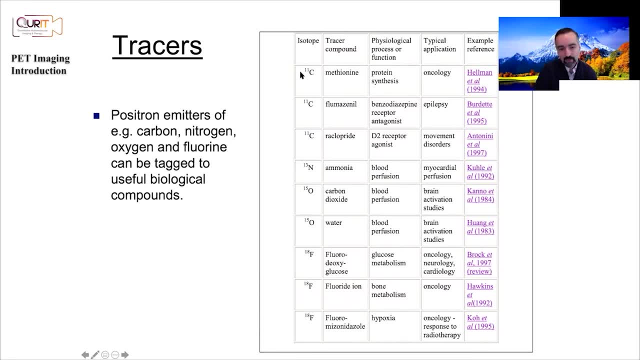 selective examples, right. So we've got four examples of four isotopes: carbon-11,, nitrogen-13,, oxygen-15, and fluorine-18.. And of course, in that lecture we gave on radiopharmaceuticals, we said that of course you could have many, many different molecules designed. 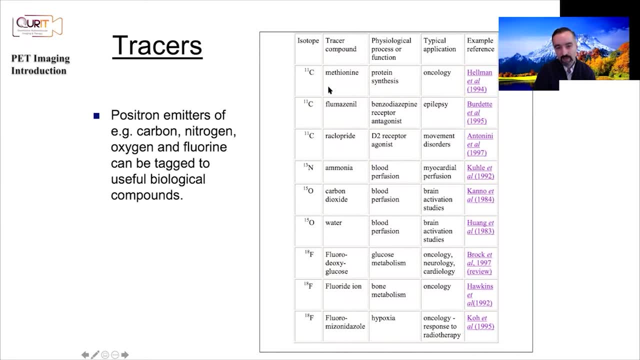 tagged with these isotopes and those molecules could be targeting different processes, different molecular phenomena. And so we've got four examples of four isotopes: carbon-11, nitrogen-13,, hydrogen-15, and fluorine-18.. And, of course, we've got four examples of four isotopes: carbon-11, nitrogen-15,. 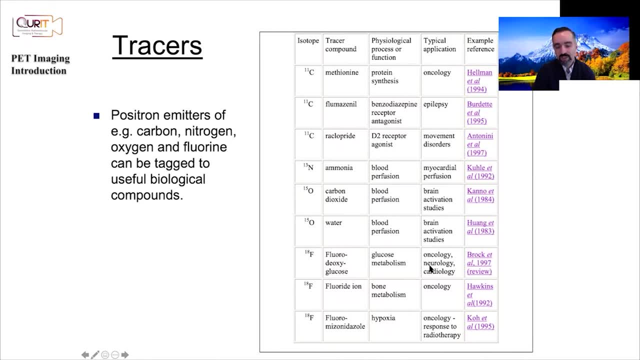 and fluorine-18.. And so we've got four examples of four isotopes: carbon-11,, nitrogen-15, and fluorine-18.. And therefore they can find applications in many different places. This is just a very, very. 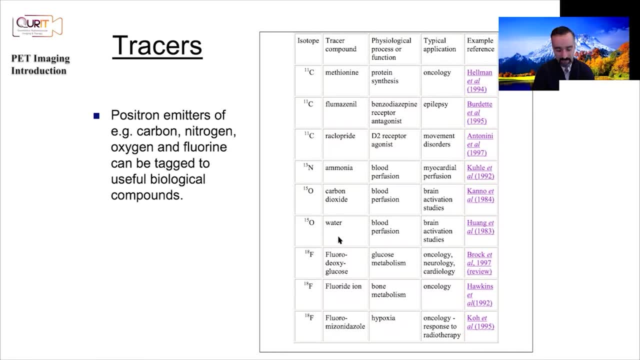 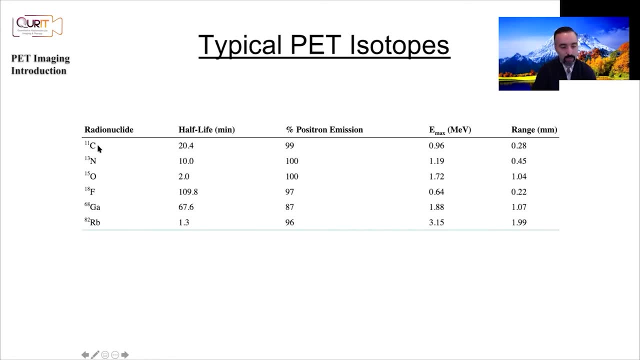 very small selection of examples right That have existed, But there is even more isotopes. So we mentioned in that one these first four, but there's also gallium-68 and rubidium-82, and there's other ones. But you can sort of see examples of half-lives We mentioned in an earlier lecture. 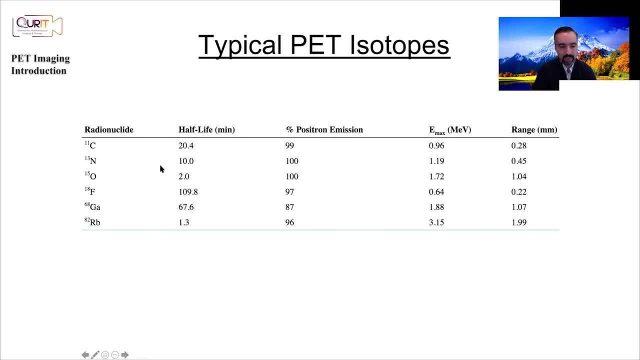 in radiopharmaceuticals that for routine clinical applications. you know, having half-lives that are way too short makes controlling the clinical environment a little bit more difficult. So that's why fluorine 18 has a good number under two hours. gallium 68 has a good number. 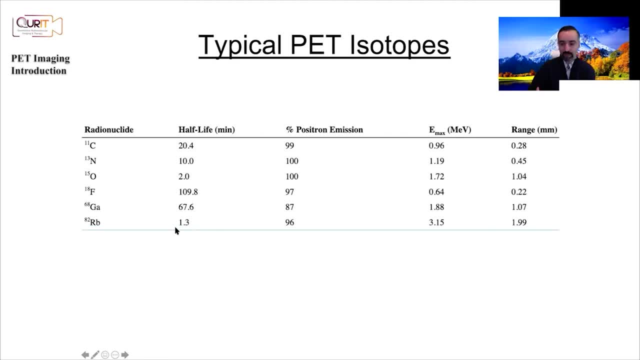 But even rubidium, even though it has a very small half-life, because you have a generator and that allows some added convenience for many, many different sites to do cardiac imaging, that has definitely found applications. So again, pedizotopes can be from different sources, from cyclotrons. 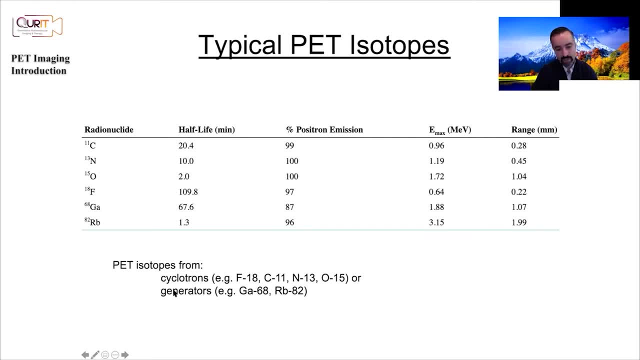 You know, in earlier lectures Carlos talked about cyclotrons versus generator approaches. But these four would be from cyclotrons, these two from generators. You know which one is better? There's a whole set of preferences and business models that are used in North America versus. Europe versus Asia versus other places. So it really depends In some sense. generator Generators have the advantage that you could have a local, inexpensive generator in your site. Cyclotrons have the advantage that you could have a sensorial cyclotron in a city for. 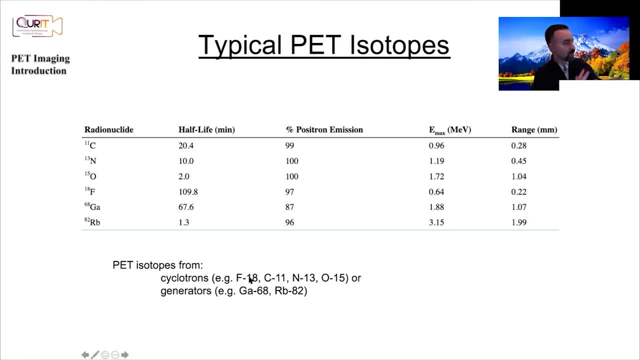 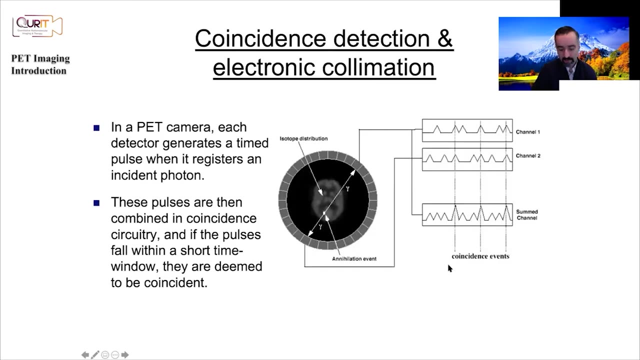 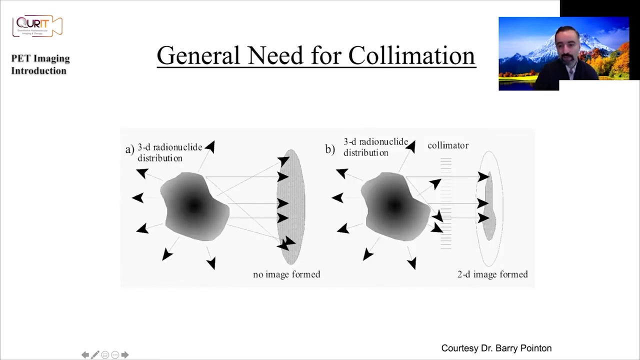 example for F18-based tracers, and it could be shipping radiopharmaceuticals to many different imaging centers. So both have clearly found applications. Yeah, So we mentioned before that. We mentioned before that Just in general. single photon imaging, if you do not have collimators, you don't know. 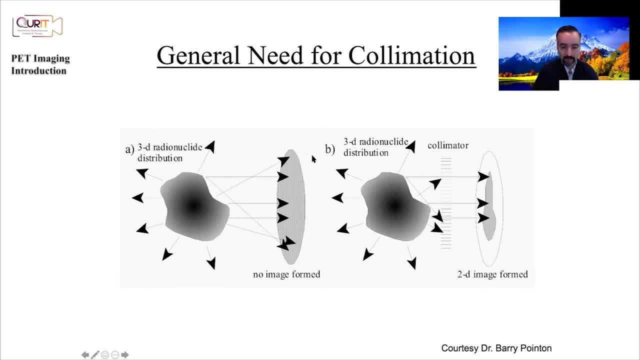 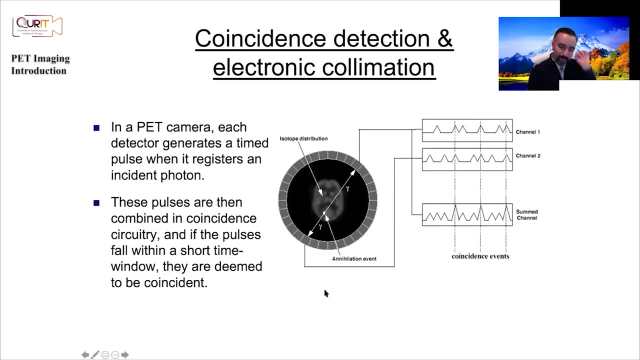 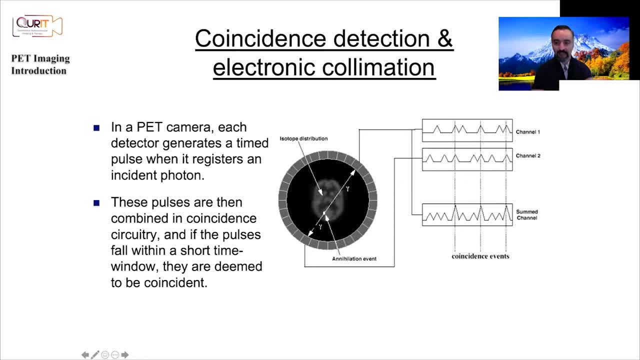 So you don't have to have a single photon imaging. So it's not single photon imaging, It's dual, anti-parallel gamma photon imaging. gamma imaging is that, you know if you've got a circuitry that tells you: well, I've got an event in one detector, I've got an. 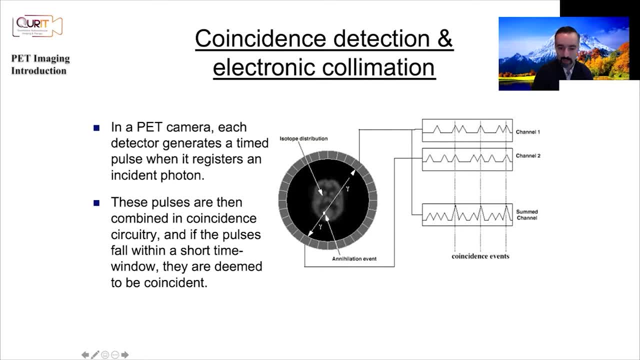 event at almost the same time in another detector. you could draw a line of response between them And you don't need a physical collimator. This is actually electronic collimation. You don't need to put a physical collimator here to ensure that only gamma rays from this. 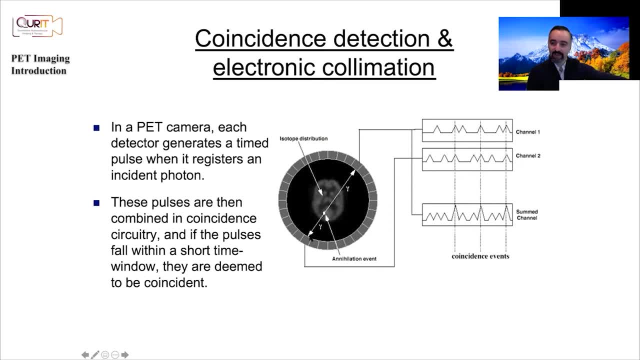 direction. Because once you know where the other, you know pair of gamma pair was detected, you can draw a line of response So you can remove the physical collimators if we're not killing so many events, And by electronic collimation you can know. 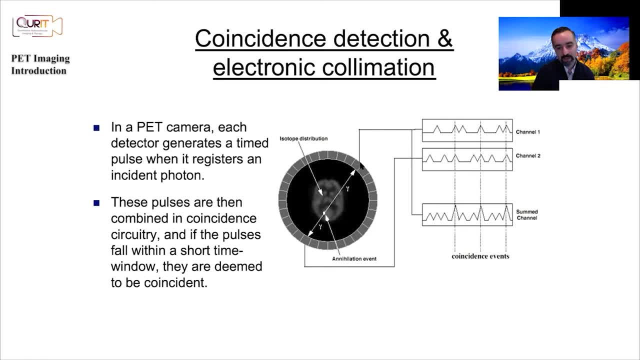 So this detector, for example, can receive events along here, here, here, here here, and they don't have to be killed, They don't have to be removed by a physical collimator, So that ends up actually significantly improving the 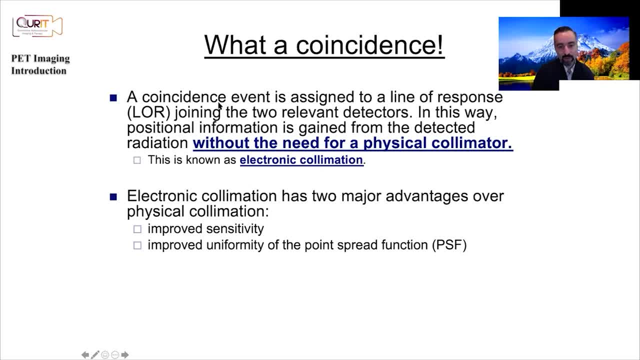 speed, Sensitivity of a PET scanner. So a coincidence event is assigned to a line of response, joining the two relevant detectors, And so you have positional information gained from the detector radiation without the need for a physical collimator. You know where the line of response, you know the direction, the angle of the line of response. 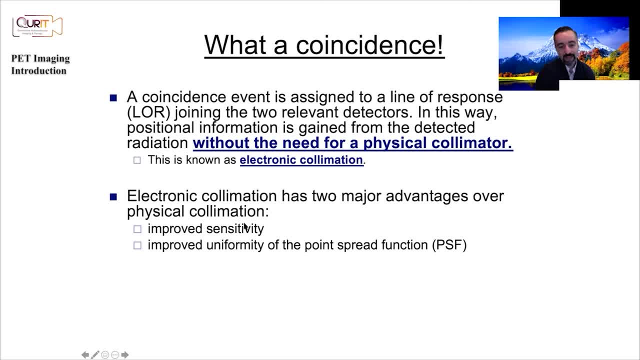 without having a physical collimator, So that results in major improvements in sensitivity. For example, compared to a typical, a typical parallel Collimator, you could improve the sensitivity by by two orders of magnitude, for example. Right, Uh, two orders of magnitude is a large improvement. 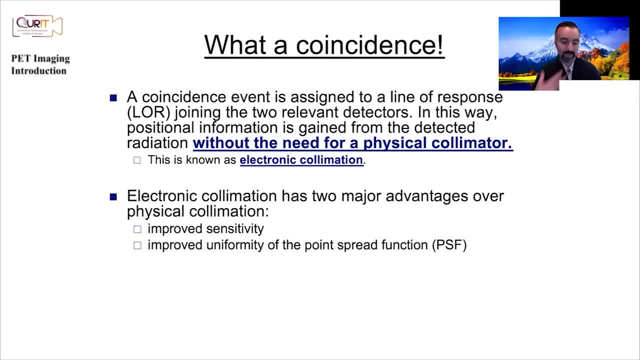 Of course, there's now been really novel collimator designs, pill pinhole collimator designs, So really, uh, the uh spec imaging world has really improved in terms of sensitivity too. Uh, and for PET, the improvement has happened by this electronic collimation. 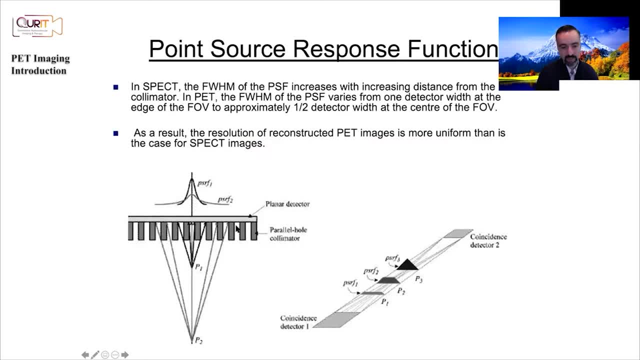 Also, it turns out, you get improved uniformity of the point spread function. Why? Because In single photon imaging, as we've discussed a couple of times before, as you get away from the face of the collimator, um your, your point spread function and your resolution. 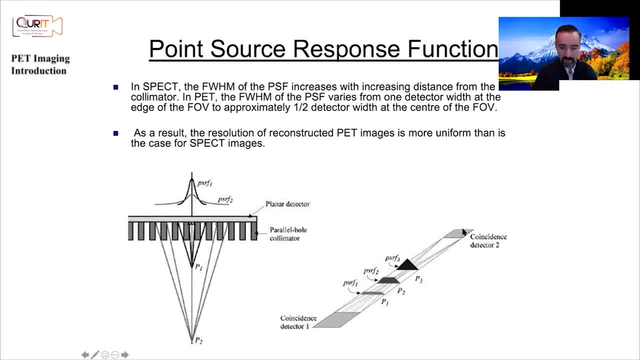 degrades comes worse, Um, but it turns out, when you have two coincidence detectors, whether you're here or here or here, sure, the profile slightly changes, Um, but at the end of the day, these are pretty similar profiles. 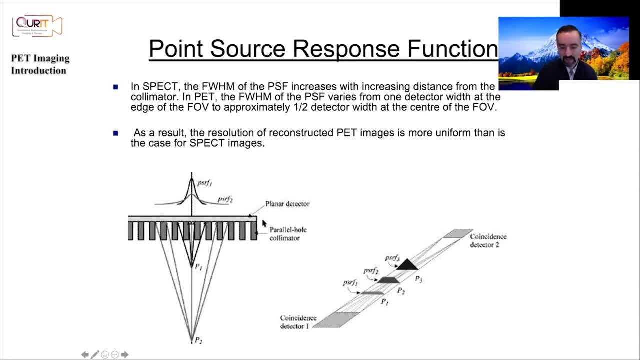 It's not like the PSF is significantly widening The because, at the end of the day, you're constrained to be within this kind of you know strip connection between these two coincidence detectors. So so there's really significant uniformity of the resolution, regardless of where you 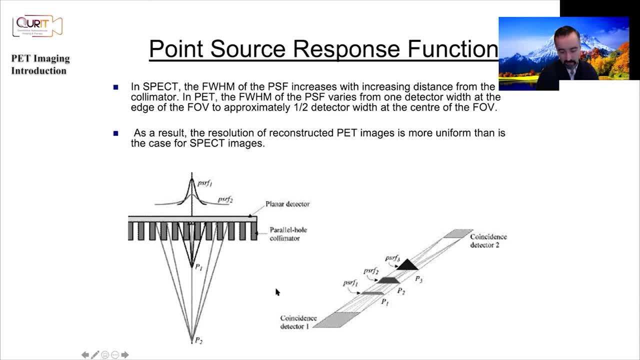 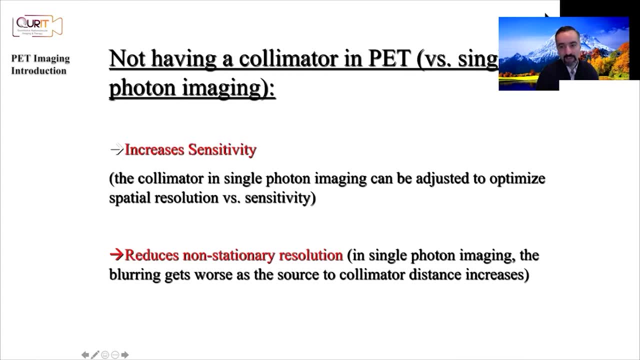 are on that line of response, unlike in single photon image. So, uh, not having a collimator, a physical collimator, in PET versus single photon, uh imaging, uh has it increased, uh it results: Increase sensitivity. 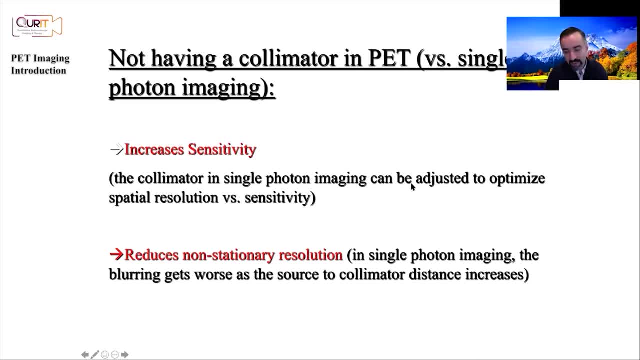 Um, of course the collimator in single photon imaging can be adjusted to, for example, improve sensitivity. But when you, for example, increase its sensitivity, then, as we've learned before, then the resolution degrades. or if you try to improve their special resolution, the sensitivity 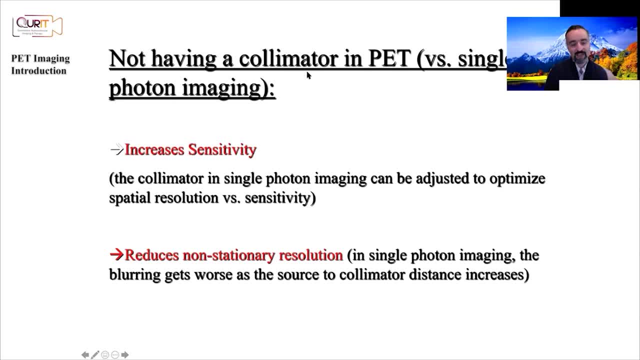 degrades. there's a trade off, Uh, but here you have a very natural way to significantly increase sensitivity in PET imaging also reduces non-stationary or depth dependent uh resolution, whereas in single photon Imaging the blurring gets poorer and worse as a source to collimator distance, uh increases. 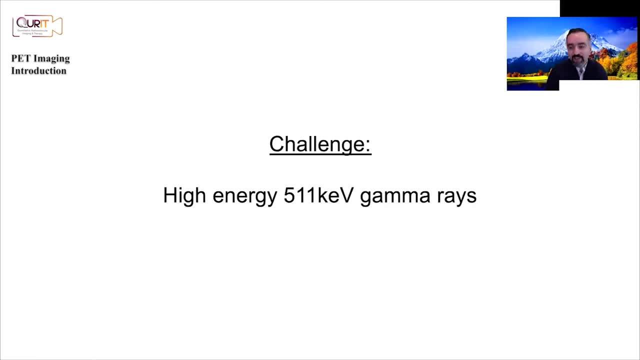 So, um, what is the major challenge with PET? Why are we then not just doing everything with PET? Why are we not just switching over? you know, to put it very simply, in a simple minded way: Well, this is so great. 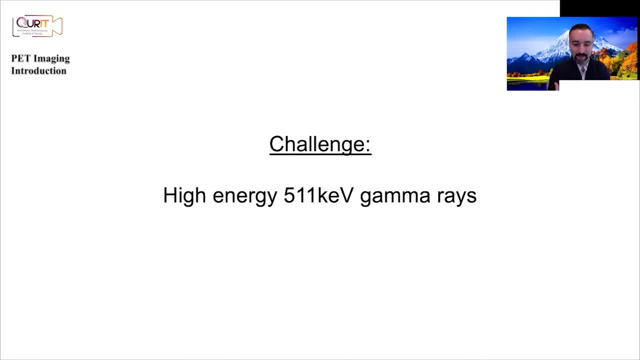 Why not just do it all the time? Well, uh, D major challenge or a major challenge in PET imaging is that, unlike single photon imaging, where the energy is tend to be definitely lower, we look at typically kind of let's say, 140 KV for technetium or let's say 208 for 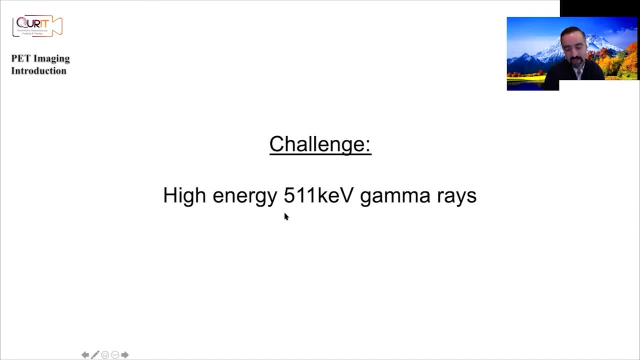 lutetium, we're dealing with far more energetic gamma rays. So stopping these and uh, you know, uh, coming up with appropriate, you know, scintillation design and all this stuff to, to, to, to stop these, it could be very expensive and could be very challenging.